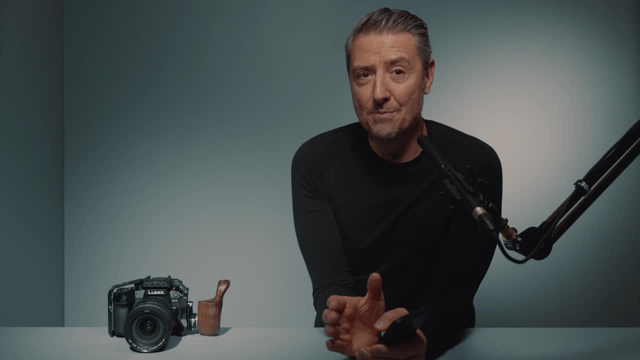 but at the same time trying to compress the file as much as possible in order to produce a fairly light file at the end. And all this happened by the magic of the codec. And remember, codec stands for compression-decompression- The codec will compress while recording. 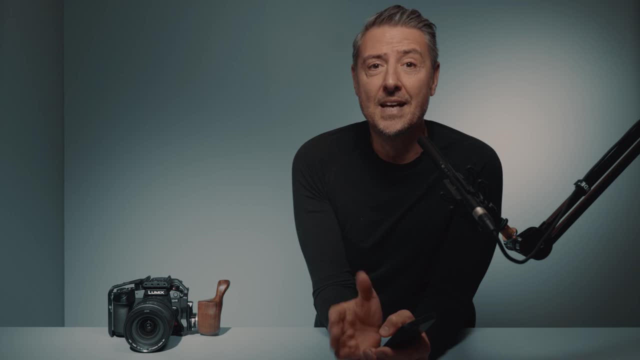 and the codec will then have to decompress while reading and editing. The All-Intra intraframe recording will record high frame one after the other. That means that every single frame will keep a large amount of information, no matter the scene and subject that you are recording. 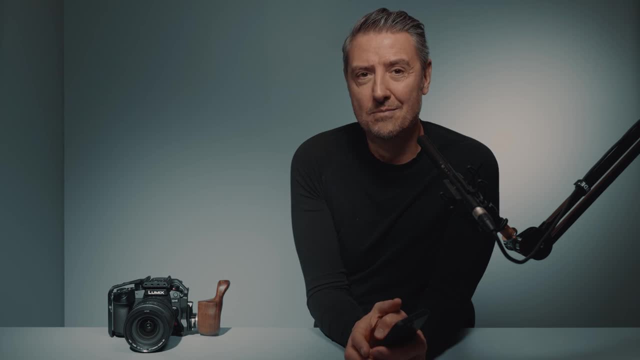 Let's take this face camera image I'm currently recording. now There is not much happening. My face and hands are moving a bit. The GH6 next to me remains still. The background doesn't change at all. So only 20 or maybe 30% of the image. 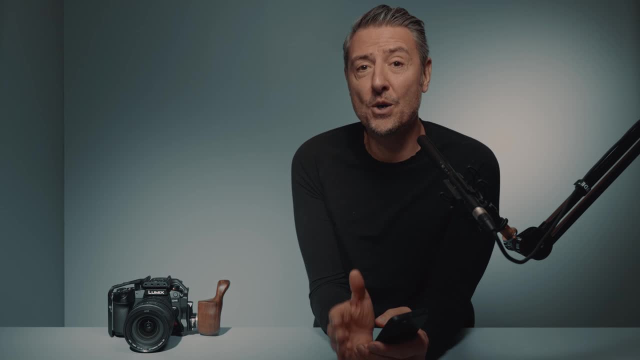 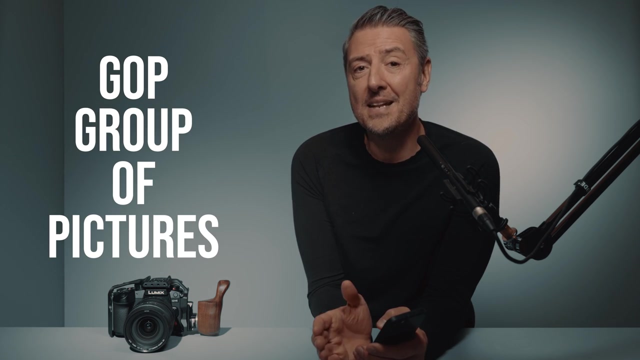 change from one frame to the other, But still, if I'm recording this All-Intra, every single frame will still keep a decent amount of information. So now back on the long-gop compression. The GOP stands for group of pictures And once again, depending on the camera and the codec, that group of picture can be short or long. 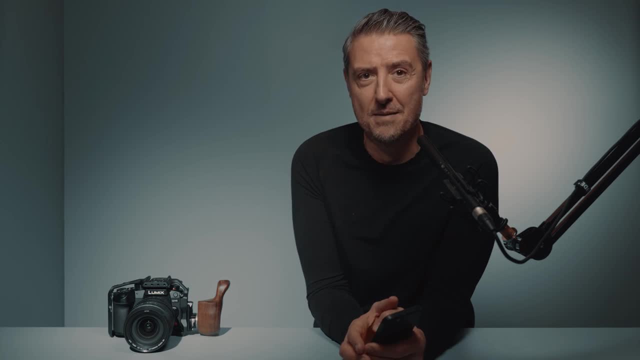 And obviously in our case it is a long G O P, a long group of pictures. We have seen that all intra recordings only capture high frame, one after the other For the long-gop compression it will also record high frame. 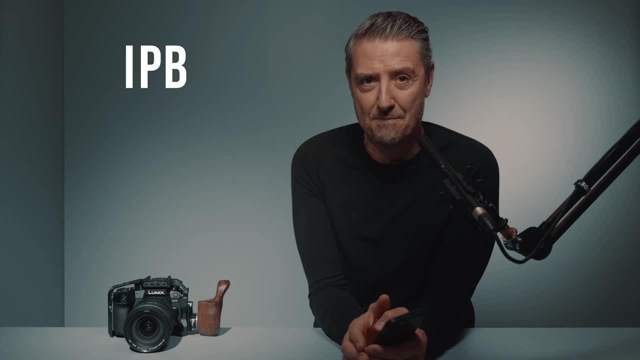 but it will record P-Frame and B-Frames. P stands for predictive and B for bidirectional, And I will not go into too much detail here for not being too long, But predictive and bidirectional frames are frames that will be created by the compression algorithm. If I step into a long-gop, it will record both the high frame and the B-Frame. B is used for the long-gop, while the high frame records the low frame, And when I go to the high frame, B is used for the low frame. 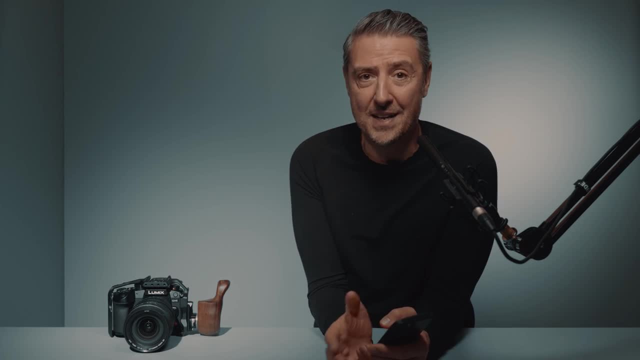 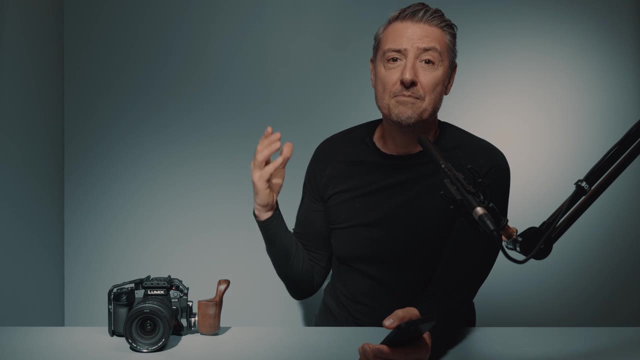 So if I go to the high frame, it will record both the low frame and the compression GOP recording for the exact same face camera setup right here. The predictive and bi-directional codec will create frames that will for sure take in consideration that many, many pixels of this. 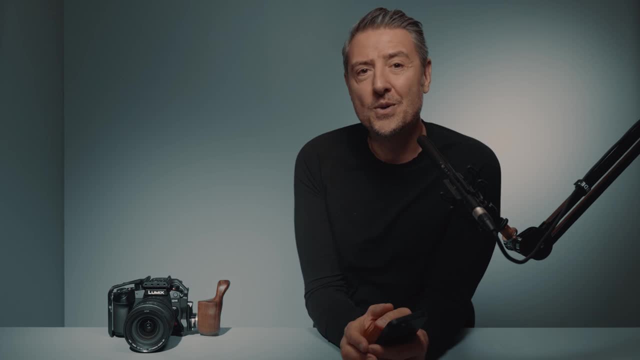 image remains exactly the same frame after frame. So instead of keeping the exact same pixel here and there, the exact same information frame after frame, as it remains the same in the background, the long GOP compression will consider recording an iframe that keeps most of the image information. 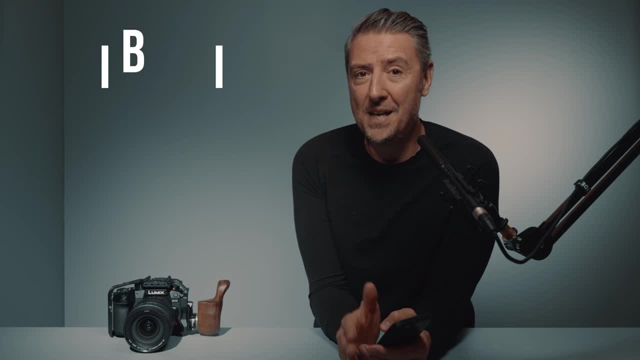 there and there and in between it will create p and b frames and those frames will only record what actually is changing into the image, basically my face and my hands movement On those specific frames. and once again, the sequence of those i, p, b frame will depend on the brand and the model. 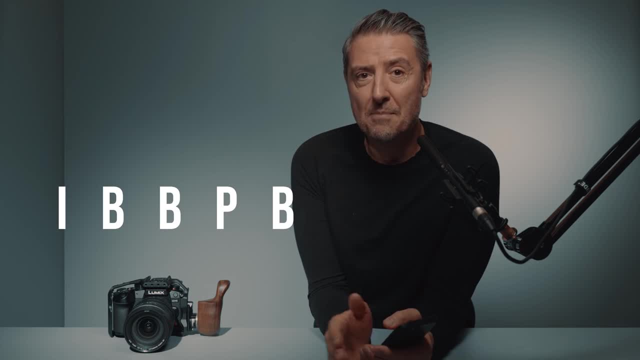 of the camera. It could look like i, bbp, bbp, bbi, so in this case this is a group of picture of 10.. By doing those long GOP compression, the camera will considerably reduce the size of the clip that you are recording. All intra recording will take three to four times the disk space. 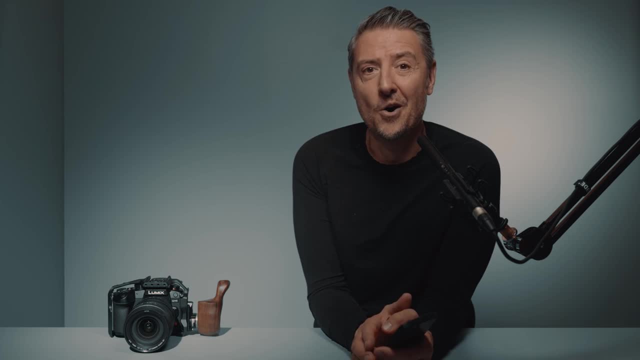 on either your recording card or, of course, on your computer hard drives, shooting after shooting. So of course, one legitimate question will be about the image quality and, honestly, it is now really hard to tell the difference in between an all intra and a long GOP clip. Has Panasonic Lumix really mastered? 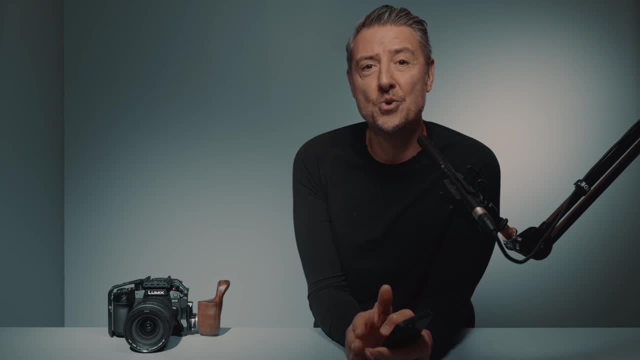 process for a long time now. I would advise you to choose in between all intra and long GOP, depending on your subject. If you are recording a complex scene with a lot of things happening in the image at the same time, like a scene with fire, water splashes or basically any scene where many things 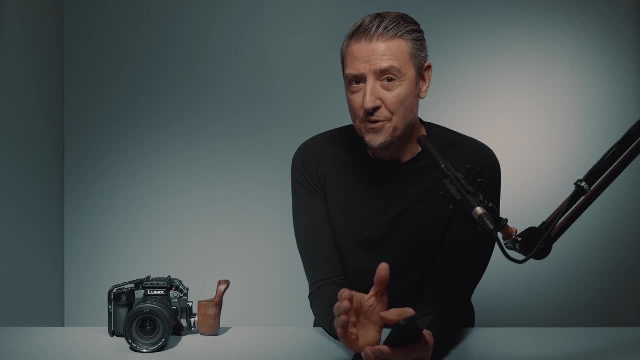 is happening on every corner of the frame, frame after frame. in this case, i would probably advise you to go for all intra. This being said, keep in mind that the codec will have to deal with that long group of picture when editing on your computer. So dealing with all intra files. 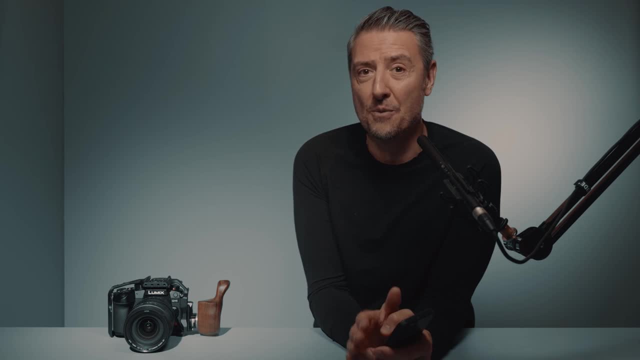 on your computer will make things much more easier for your computer CPU. This is so true that it is recommended sometimes to convert the long GOP files into a proxy all intra file in order to edit smoothly on a weak CPU computer. So you will have to keep all this in consideration. 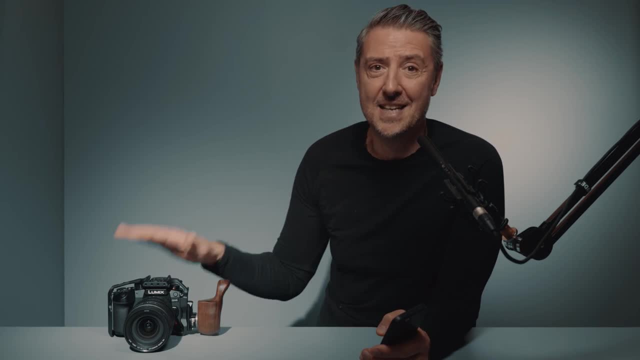 when choosing the recording format, and there is a lot of them inside the GH6. And once again, Lumix did things really well here, as you will be able to filter all those recording settings based on any of your preferences. Imagine that you want to see only the all intra recording.